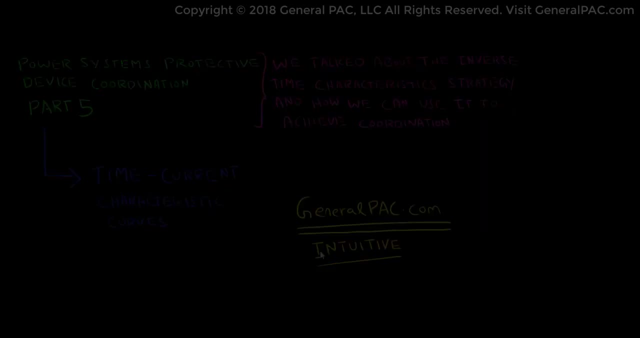 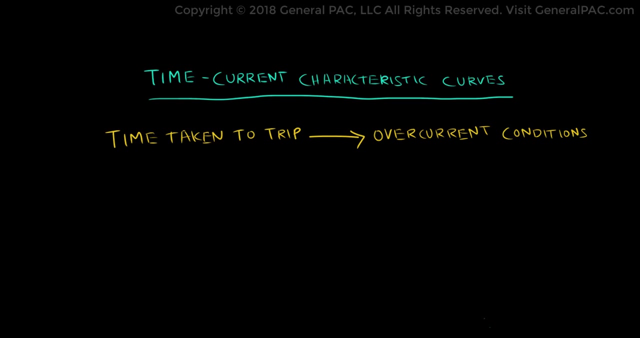 Our goal is to make power systems intuitive. Time current characteristic curves are used to show the time taken by the breaker to trip for a range of overcurrent conditions. They define the operating characteristics of a protective device. The x-axis shows the current level and the y-axis is used to show the time taken by the protective device before the trip in action is initiated. 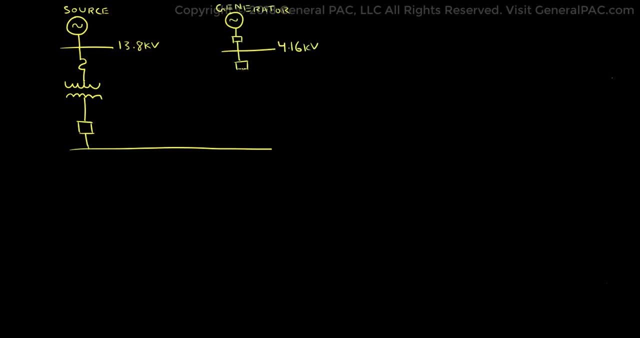 To explain this concept, let us again consider a facility with a 50 kVa, 60 Amps static load, As discussed in Part 4, we will be discussing the time characteristic curves In previous parts. all breakers should be rated at some percentage above the full load Amps of the downstream load. 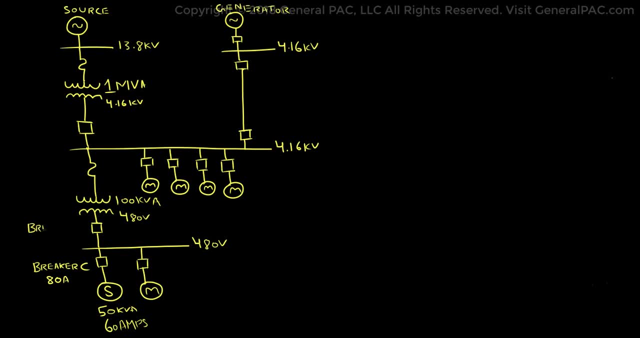 Breaker C is rated at 80 Amps at 480 V, Breaker B is 120 Amps at 480 V and Breaker A is rated 100 Amps at 4.16 kV. The breaker Amp rating is much greater when we compare all the breakers at the same voltage level. 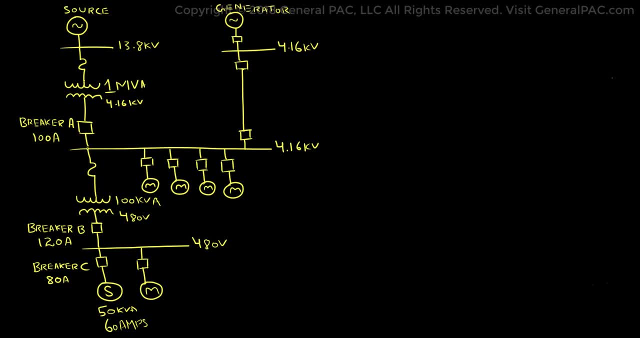 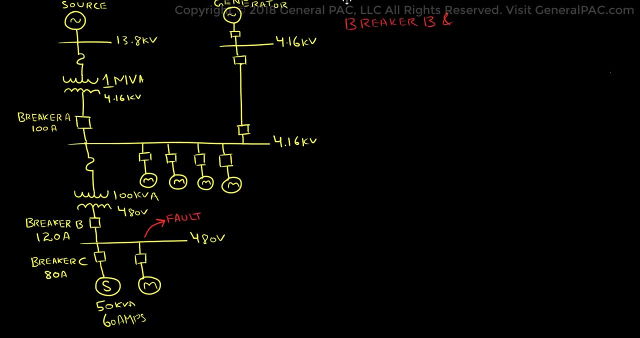 To demonstrate how time current characteristic curves can be helpful in achieving coordination. let's consider a fault between Breaker B and Breaker C. For this case, let's assume both breakers to be thermal magnetic breakers. We will now plot the curves of Breaker B and Breaker C on the same axis. 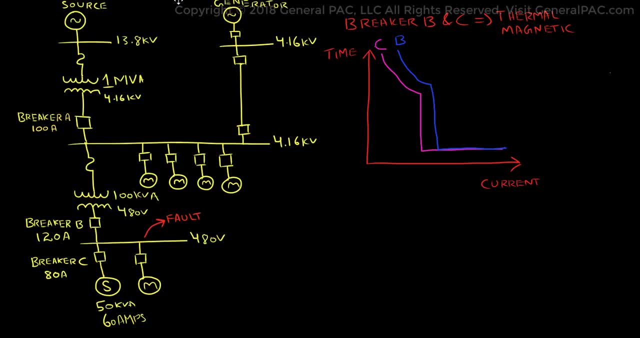 We can see that Breaker B picks up at a higher Amp value, while Breaker C picks up at a lower Amp value. This results in a shift between the curves and allows coordination. Now that we understand the basics, let's go into more detail and talk about the circuit. 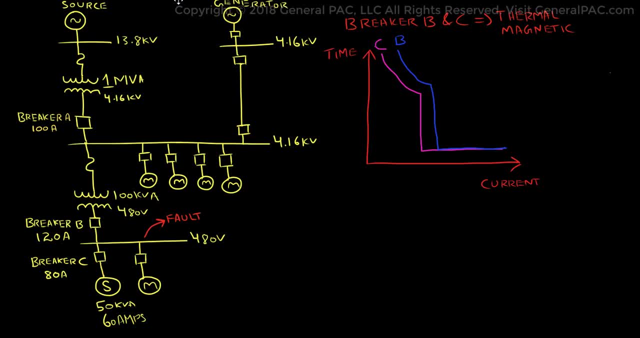 Now that we understand the basics, let's go into more detail and talk about the circuit. Let's look at the different regions of a time current characteristic curve For a thermal magnetic breaker. there is a long time region which starts from the pickup Amp value. 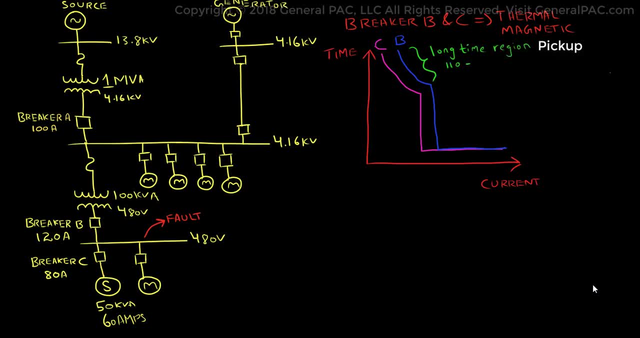 This region includes the protection against overloads from 110 to 120% of the Amp rating. There is a fixed, non-adjustable time delay for each breaker, after which it enters the instantaneous region. This instantaneous region could begin from 200 to 300% of the Amp rating. 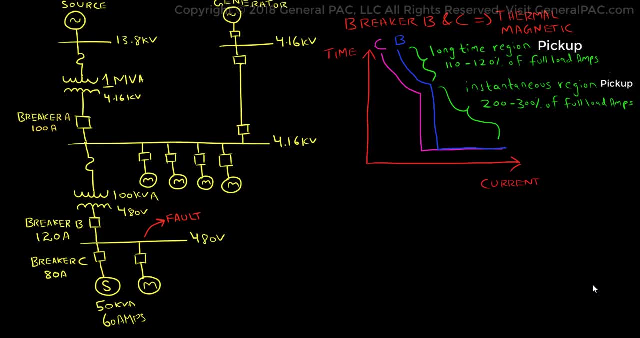 And is used for protection against high abnormal currents. The instantaneous region has a very small delay of a few cycles, After which the tripping action of the breaker is initiated. This is one way of achieving protection coordination using inverse time characteristics and the breaker-Amp ratings.